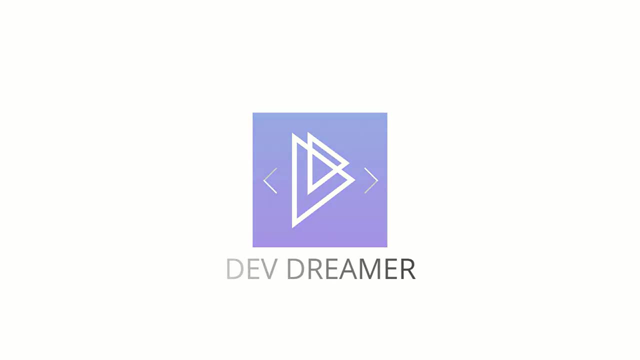 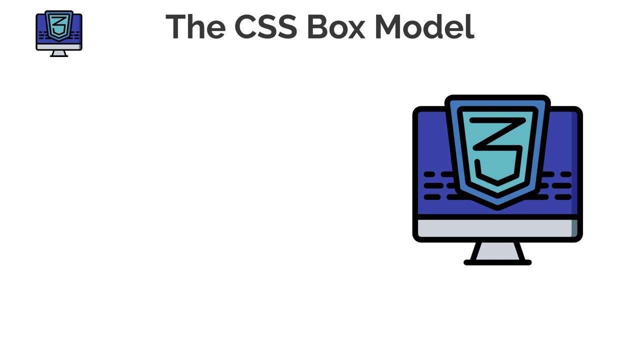 Hey there guys, it's Amit, and welcome back to DevDreamer. Now, this is a very important lesson, because this is all about the CSS box model. Now you might have heard this before. people say, oh, the box model, and you know you might think what is that? Well, the box model is actually the core. 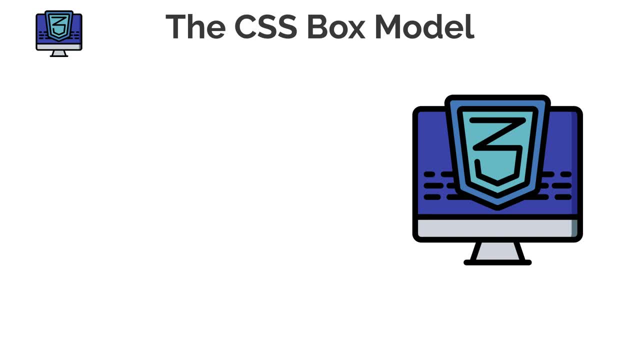 of understanding how our elements are laid out on the screen and how different CSS properties affect different elements as to their layout. Essentially, you should think of every element as having a box around it, hence the term box model. So pretty much every element consists of. 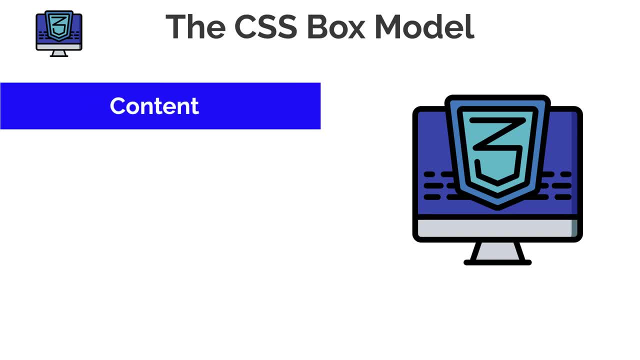 the following. We have the actual content, so it could be a paragraph, element a, h1, a div, whatever right. Then we have the padding. we looked at padding. remember padding was inside. We had padding inside margin outside. Remember that good old acronym PMOL, which means nothing but everything. 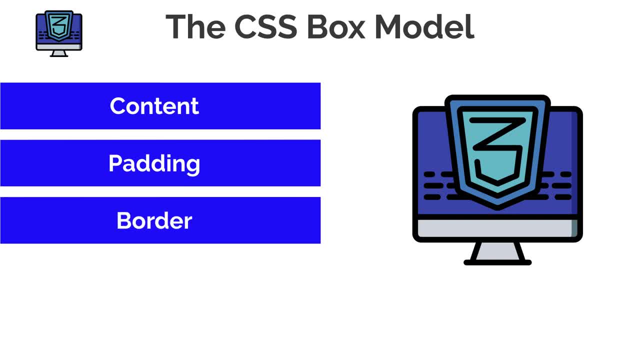 at the same time. Then we had the border, which goes around our content and padding, and then, finally, we had margin, which goes outside of our border. Okay, so we've got content, padding, border margin. Let's take a look at it in a bit more detail. 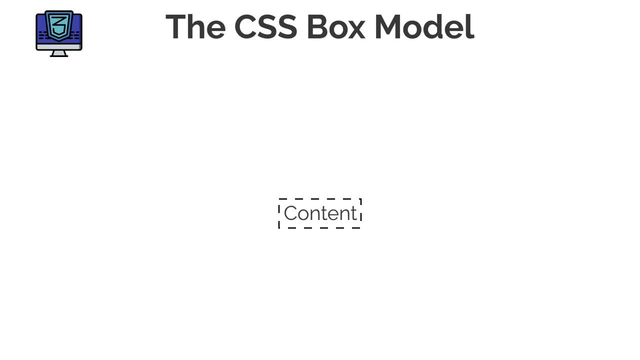 So this is the content, and again, this could be a paragraph element, a div, whatever, and then outside of that, then we have the padding. Now, I shouldn't have said outside. essentially, what we mean here is that we're increasing the spacing between the content and what would be the border. 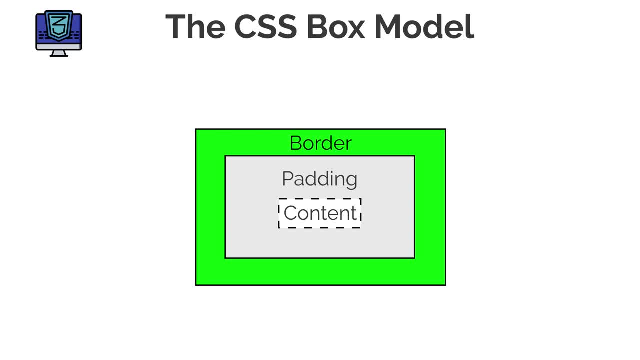 So here, then we have the border- okay, that goes around the padding and the content- and then, finally, we have this margin, which is the spacing and area outside of our content. So this is the content and again, this could be a paragraph element, a div, whatever. 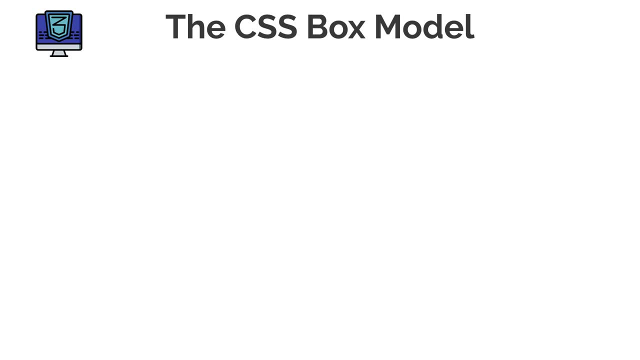 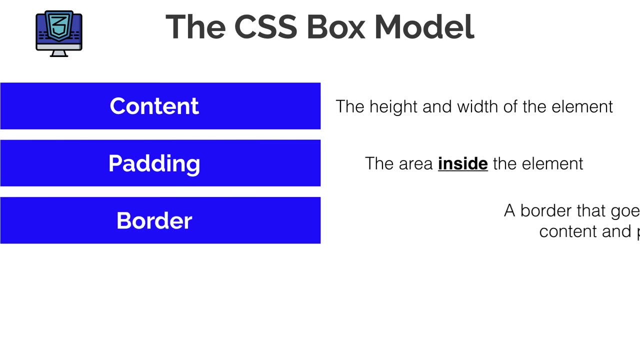 Okay, outside of the border. So to recap, before we look at an example: content is the height and the width of the element, padding is the area inside the element, border is a border that goes around the content and the padding and, finally, margin is the area outside the element. 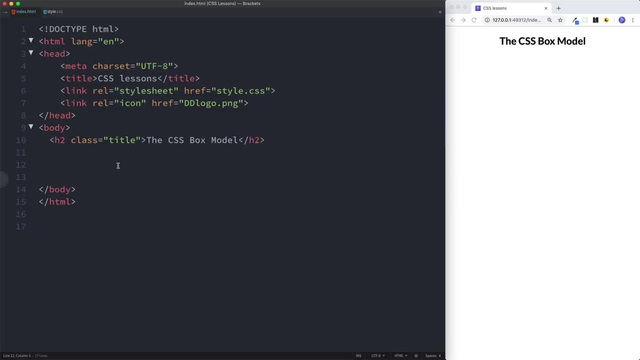 Okay so, now that we know all that, let's take a look at an example. Okay, so here we are, then, in our text editor. Now that we have a basic outline and overview of what the box model is, let's take a look at it in a bit more depth, with some examples. 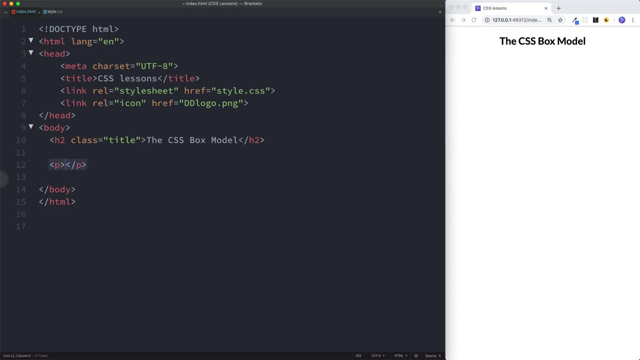 Okay. so first of all, I'm just going to put a paragraph tag here and let's just say: dev dreamer. Okay, let's head on over to our starcss file and here the first thing I'm going to do is I'm actually going to give this a. let's give it a caps lock first. okay, I'm actually going to give 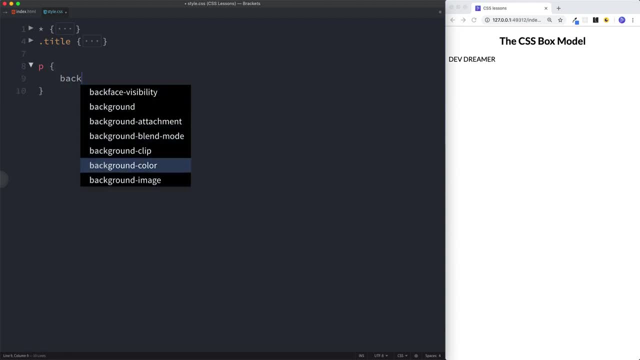 this a background color, So we're just going to say background color and let's just say sky blue. Okay, this is going all the way because it's a block level element. Let's just change that by doing display inline block. Okay, let's just change that by doing display inline block. 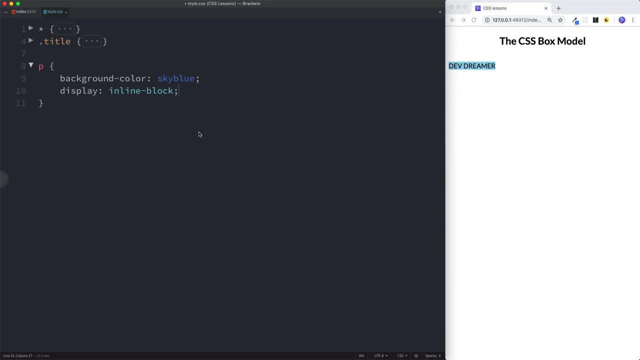 Okay, let's just change that by doing display inline block. Okay, let's just change that by doing display inline block. To learn more about what this is, I will leave a link on the screen somewhere or in the description box below, And let's also say: let's give this a padding. Now, if you've been following along with, 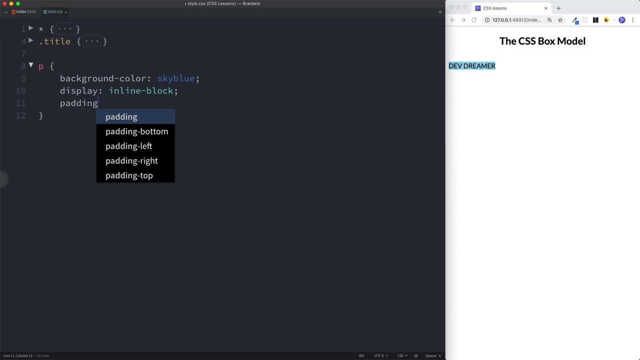 these lessons and you're actually going through the playlist. you should now know what padding is and the different ways in which we can apply padding: Padding bottom, left, right, um, declaring on one line, etc. etc. Okay, and you should know what this will do as well. 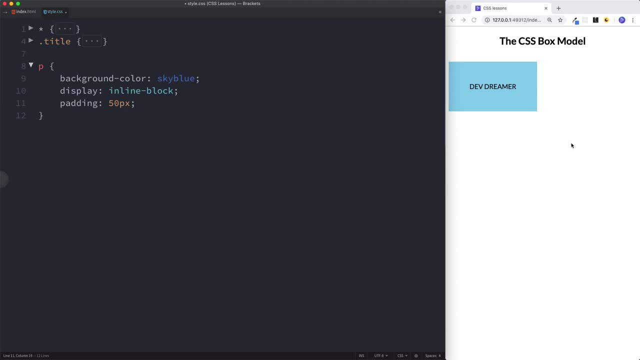 So if you do 50 pixels, yep, this increases the space Inside of our element. Okay, let's give this a border as well. Let's say 10 pixels solid. Let's go for this lime green color. Let's also now apply some margin to this as well, So let's say margin top. 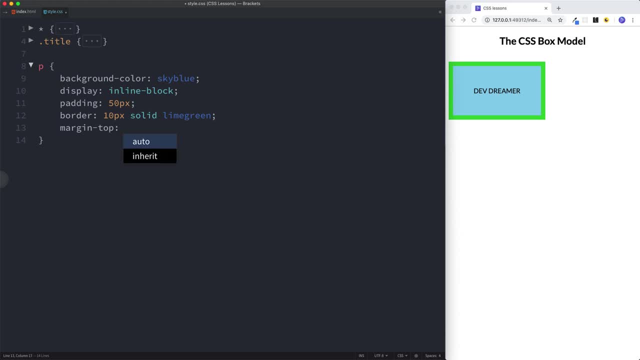 because you want to move it down from the top here. Let's say margin top 150 pixels, And what that does is it increases the spacing here at the top, margin top by 150 pixels. Okay, that's why it's been pushed down here. 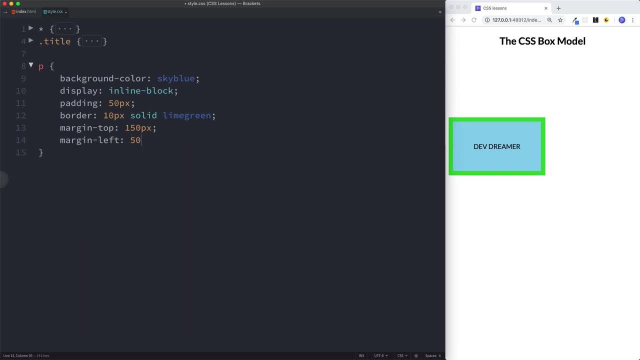 And I'm also going to say margin left of, let's say, 50 pixels. Okay. so that's moved it to the right, pushing it from the left, Okay. so our element then now consists of the content, of course- padding a border, as well as margin. Now, if you're using Google Chrome, I know that some 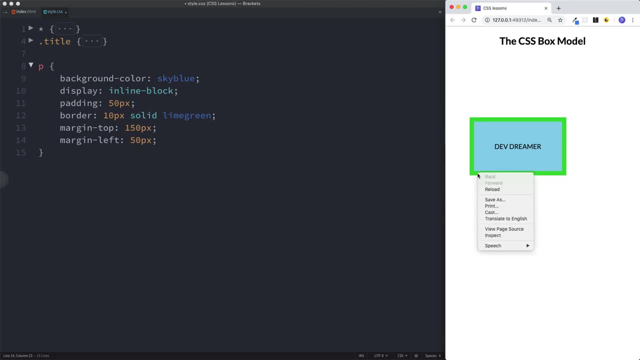 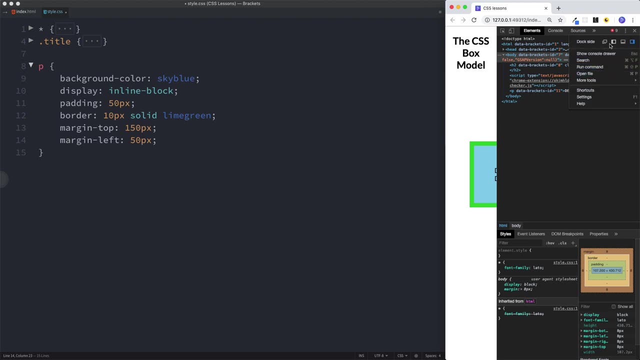 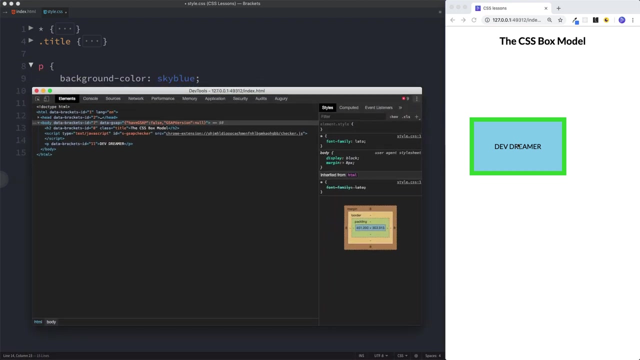 of the browsers do this as well, but if you're using Google Chrome, you can actually right click the page and click on inspect. This brings up the Google Chrome developer tools. Let's actually move this So you can just say: check it out. let's just keep it here for now. Now, as you're building sites and 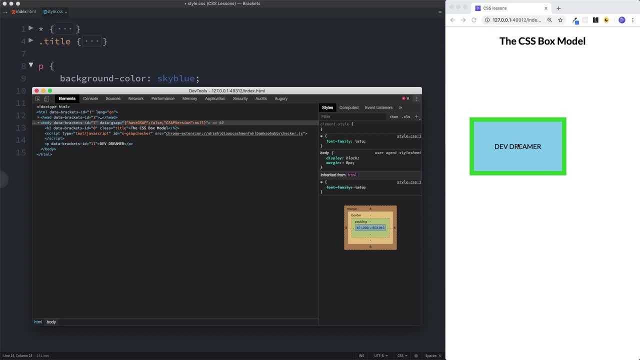 you're working on projects, you're inevitably going to be using Google Chrome developer tools. It's just so helpful you're gonna find yourself reaching for it a lot Now within the computed section here. okay, We can actually see we've got this diagram, and this diagram represents: 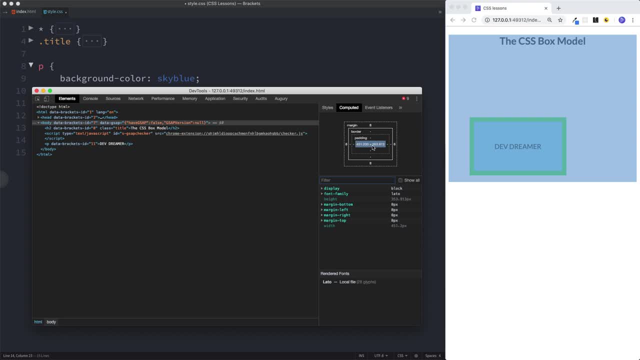 our element. This blue area here represents the content, This represents the padding, This is the border. Okay, the margin, which is not right. let's see why. that is okay. so that's, that's the actual body. so this is our HTML here. so it's actually selecting the body we want. 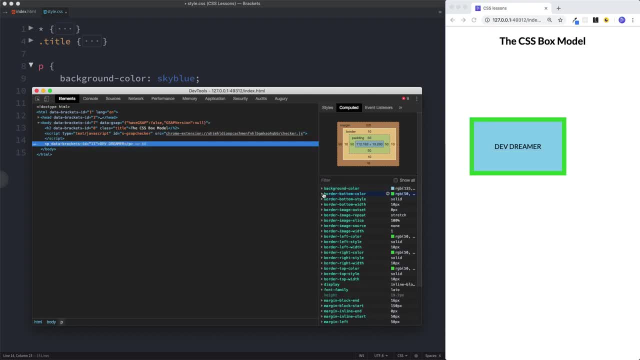 to select our paragraph element which is right here. okay, that's like this, right? okay, this is the content. as you can see. it's highlighting what that is. in this case, it's just our paragraph element of dev dreamer. okay, this is the padding. just zoom in here. in fact, what I'm going to do, I'm actually going to change the. 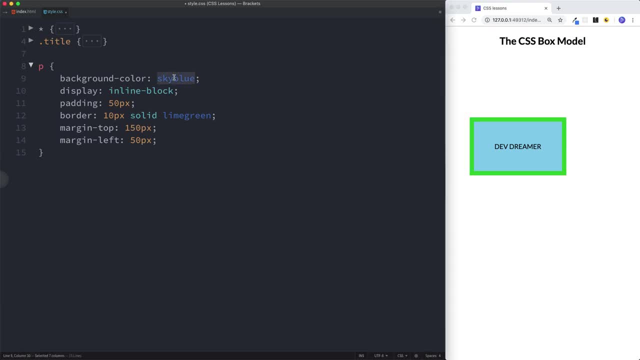 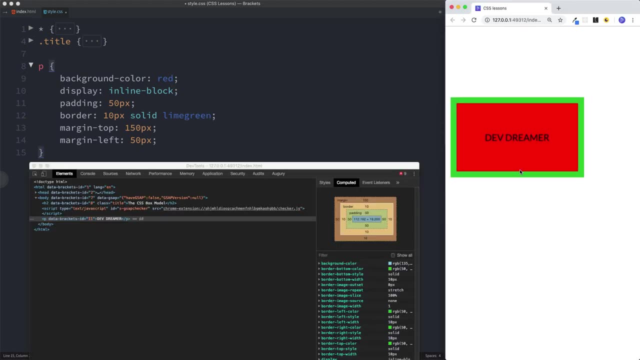 color of this here. so nothing that helps, let's go for. let's go for red, okay. hopefully that'll be a bit easier to see. just zoom in as well, okay. so again, this is the content, this is the padding, this is the border and this is the margin. 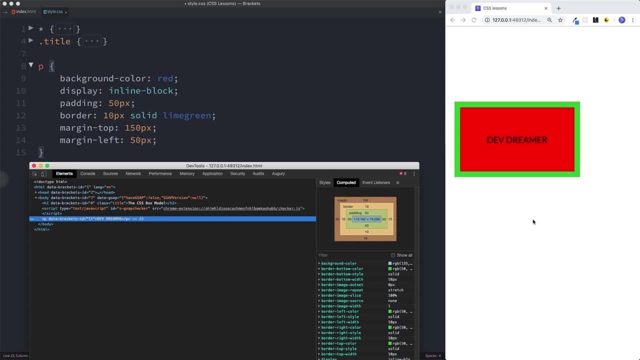 okay. so once you understand then that every element is a box, you can then start to think about how you want to lay them out, because let's say, we had another element here, let's just go to this and go back to our HTML file. let's include another. 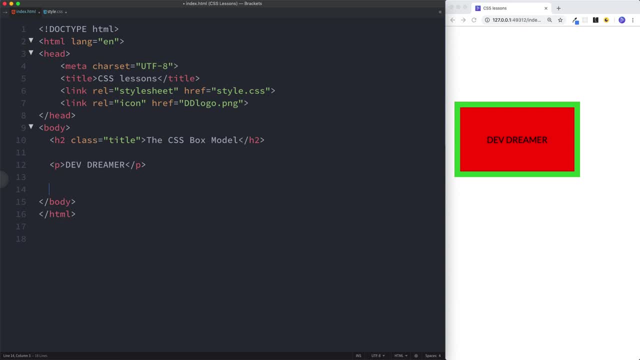 element here. it's going to be a. let's just put a h3 that just says hello there. okay, we've zoomed in so we can't see it. there we go now. first of all, take a look at where it is. why is our h3 all the way down here at the bottom of the page and 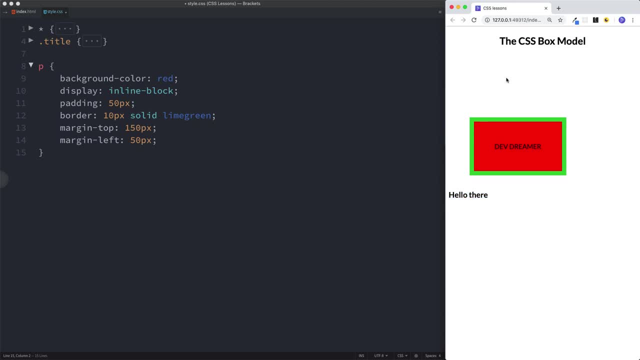 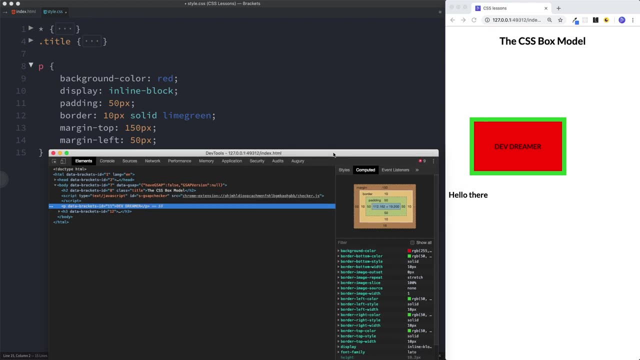 not appear, that's because it's being affected itself by the styling that we applied to our paragraph element. okay, so if you right-click and inspect- in fact don't need to, we're already in it- and let's select our h3. not only does our h3 have its own styling, because the 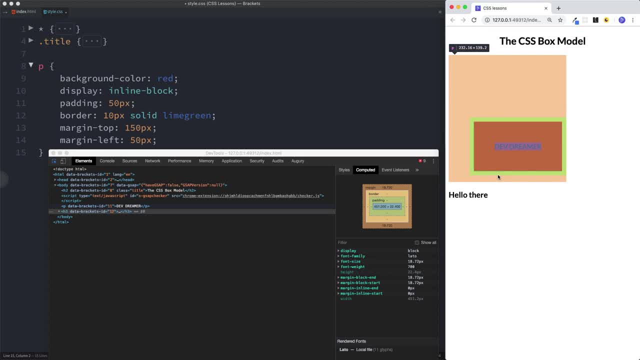 default browser styling. but also if we hover over here, we can see that this- I'll use it on here- actually be easier paragraph. okay, right here. if you look at the very bottom, you see that this is where the new styling for our h3 begins. okay, so ends about there and then it starts again here. now let's say we 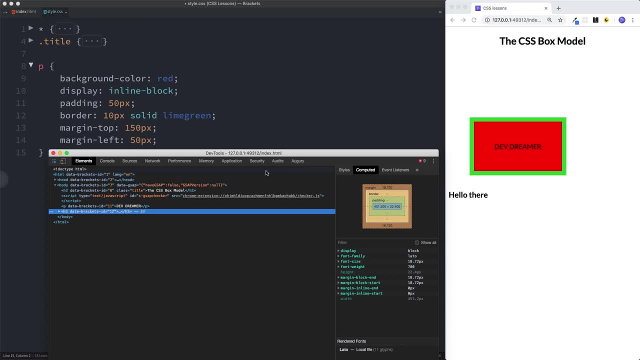 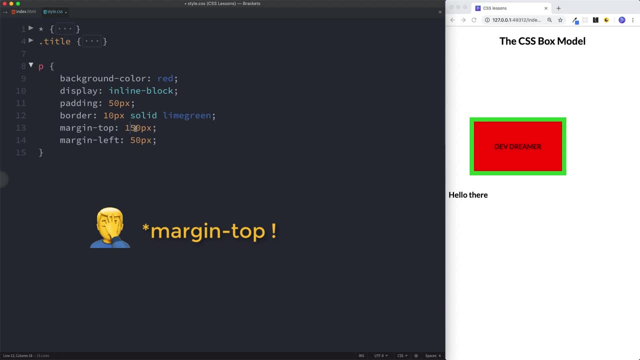 didn't want it to be further down here. let's say we want to all our elements to be pushed up. well, what we can do then let's go do this now. what we can do is we can actually reduce the padding on the top. here we can say padding top, let's just say 50 pixels instead. okay, that's. 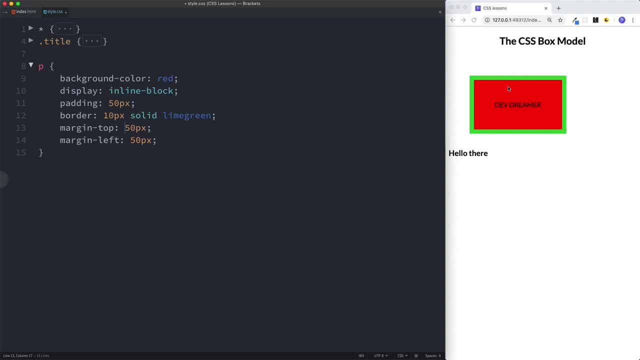 all moved up. it's not only our paragraph element that's being moved up, but it's also our h3 element. okay, and let's say I wanted to keep our paragraph element where it is. I only wanted to move by h3 down a little. so up here let's say h3. 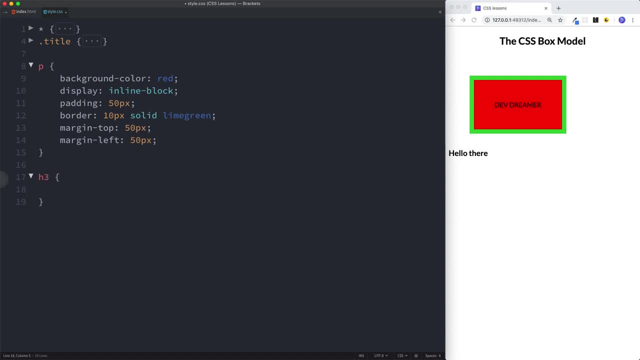 H3 and let's increase in fact, before I say it, what do you think we should do? we want to do now is remember that we've put unpack the his case because it's not DIRECT. Serge Keeley and laptop designer, get personality. you're primary eBay, okay, well, and let's say here, let's say h3 and this increase in fact, before I say what do you? 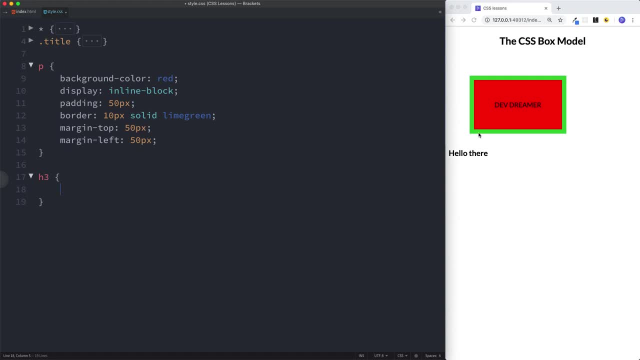 think we should do. we want to move our h3 down a little, so we've got some spacing between the two, between our two elements. what should we do? what do you think? well, we need to apply spacing outside of our element because we want to create some space and some distance between our two elements. so we'll just 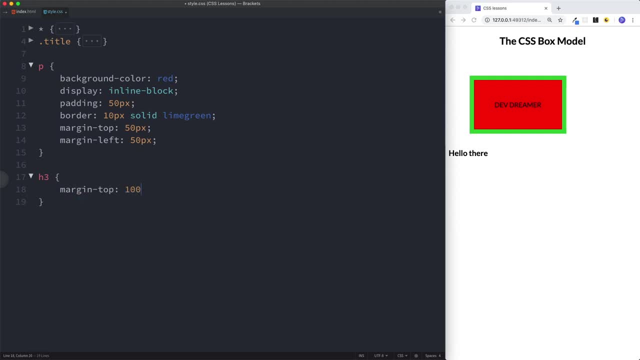 say margin top, let's say 100 pixels. okay, and that's moved it down. now there are going to be some other things that affect this, such as positioning, but for now, practice this with your own elements and have a go at laying them out. and there is one thing, actually, I'll leave you with, and that's all about how. 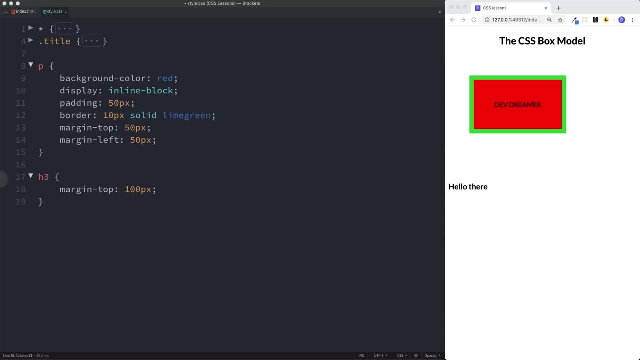 to apply width and height to an element. let's say we wanted a paragraph element that was exactly 300 pixels wide. okay, let's get rid of all this, and I'm gonna get rid of this as well. okay, and let me just delete this h3 as well, because it's. 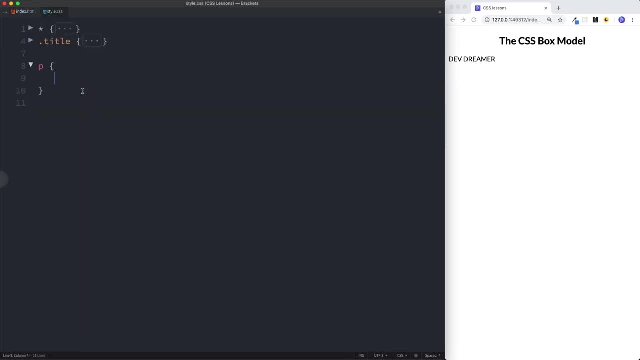 just in our way, okay. so here then I'm going to say: border, one pixel, solid red, and also, let's just say display inline block, okay. and now I'm going to say: I want this paragraph element to have a width of 300 pixels. now question: does our paragraph element have a width of? 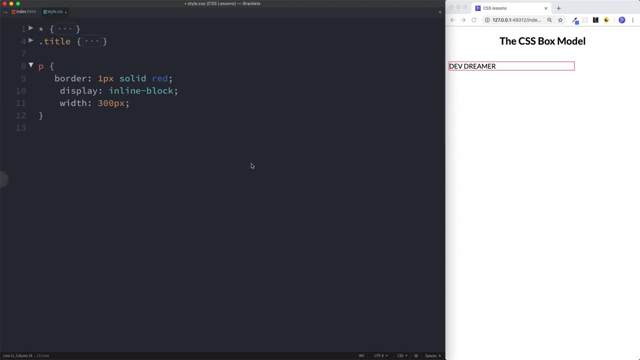 300 pixels. have a real think about it. what if we were to also say we want to put some padding on here, let's say padding of, let's just say, five pixels all the way around? okay, and also it's too close to this side here I actually 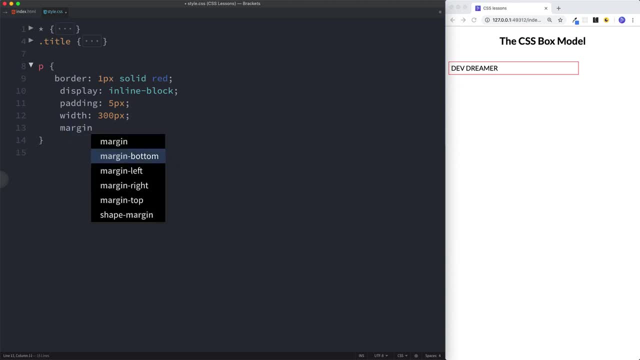 want to. I just want to move this out. so let's say margin, I've been left by 10 pixels. just on the left, though, and finally I'm just gonna say text align: Center put into the middle. okay question: does our paragraph element now have a width of 300 pixels? 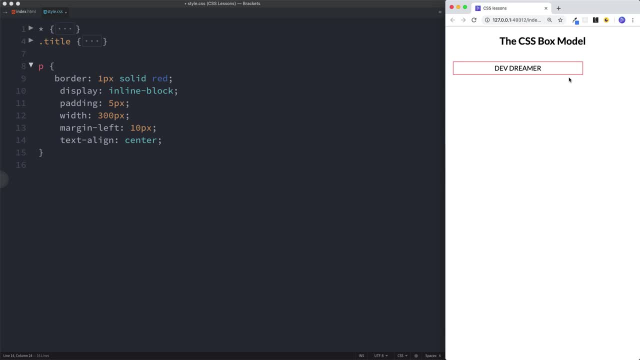 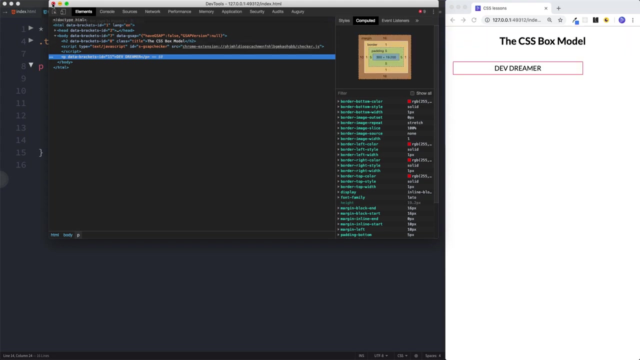 well the answer. it was a bit of a trick question. the answer is yes and no, because if you're referring to just the content of our paragraph element, then yes, that does have a width of 300 pixels- okay, 300 pixels. however, our paragraph element no longer simply consists of just the content. 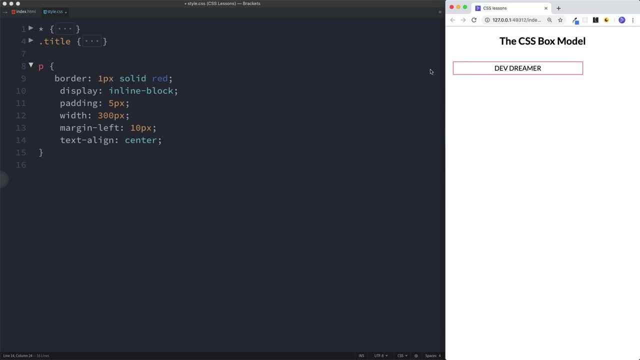 because we've also got a board of one pixel going all the way around. we have padding of 5 pixels, margin left 10 pixels, So actually our paragraph element, the whole thing has a total width of, so content was 300 pixels. plus we had a one pixel border going all the way around, so one pixel here. 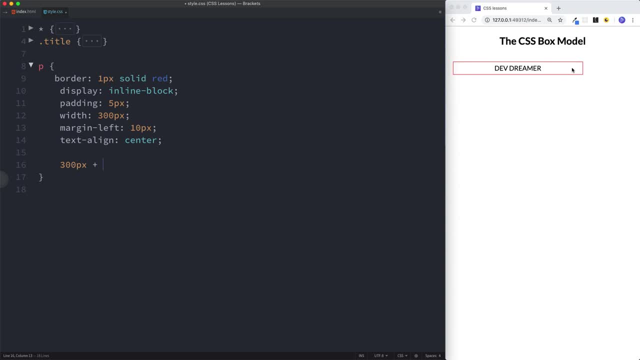 and one pixel here, okay, So it's going to be one pixel plus 300, plus another pixel there, so it's going to be plus two pixels, okay, One pixel here and one pixel there, plus the padding of five pixels going all the way around. 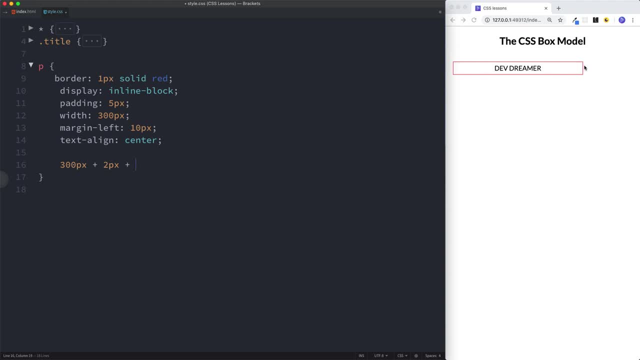 so that's going to be five here on the left and five here on the right. Remember, we're just looking at width, we're not looking at the height. so padding top and bottom and boarding on the top and bottom, we're not interested in that in this example. 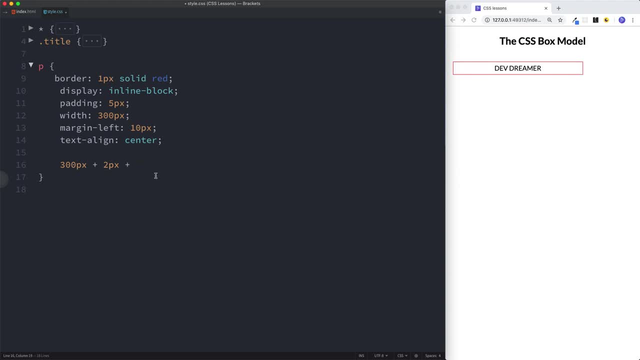 So we've got padding on the left of five pixels, padding on the right of five pixels, that's 10 pixels altogether, okay. And then finally, plus margin left- 10 pixels okay here. Now, if we only have margin left, we haven't specified margin all the way around and there's. 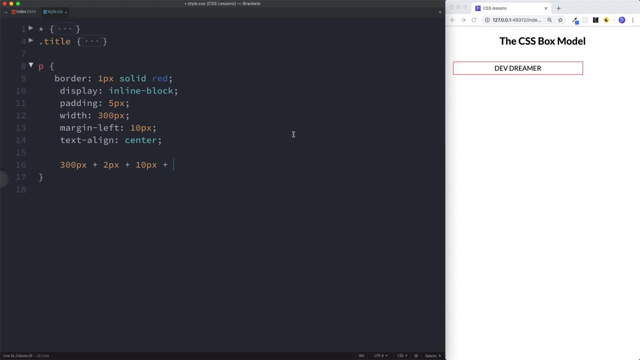 no margin on the right either, so this just has a margin left of 10 pixels. okay, so 10 pixels, So 10 pixels. So the total, The total width of our element, is 322 pixels. okay, Okay, guys, so go ahead and try this yourself.